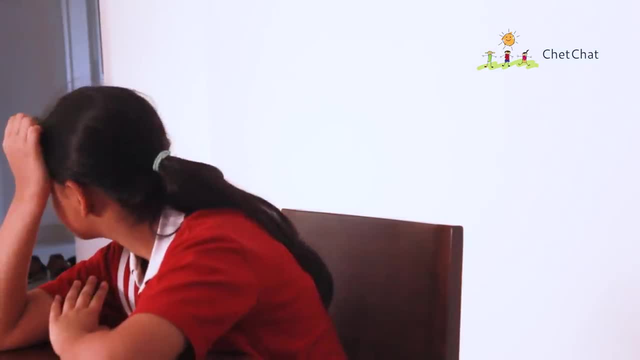 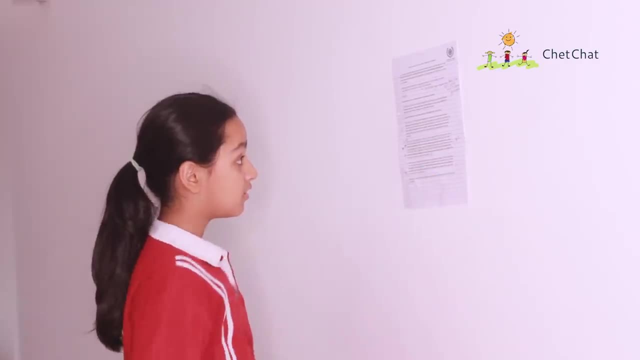 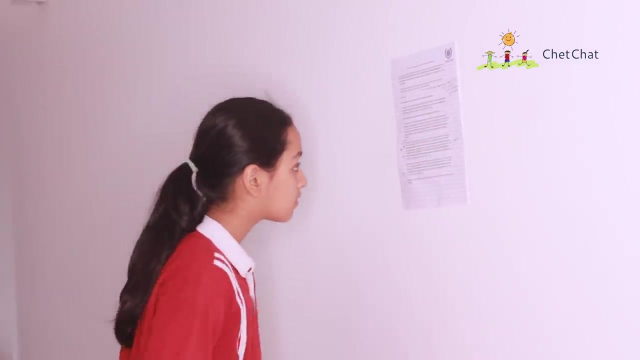 has to give a live presentation of two math topics in front of the class. She couldn't believe her ears, but she had no choice. According to the notice on the board, she got probability and angular relationship as her presentation topics and unfortunately she dreaded both the topics. Lavanya couldn't sleep at night. 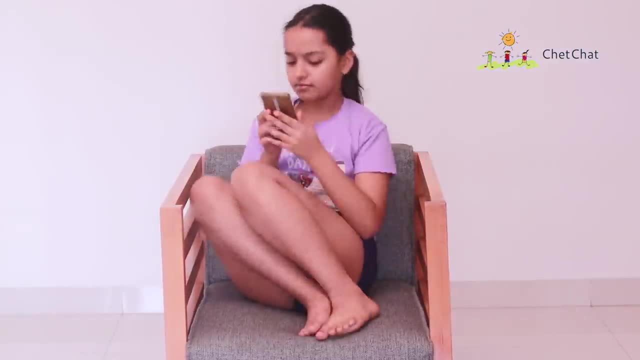 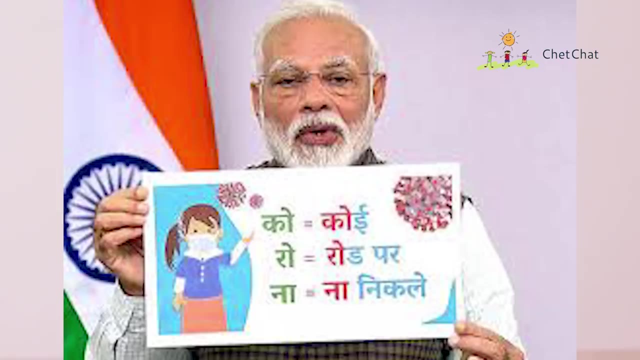 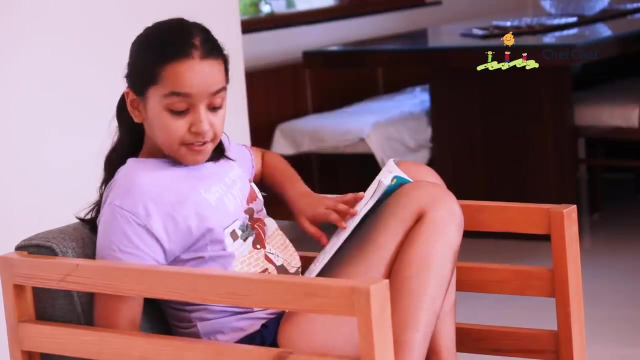 Luckily for her, a few days later, another announcement dropped in by the principal. This was regarding the nationwide lockdown announced by the government as a safety measure to a global pandemic. She was super excited that the presentation is going to get cancelled, But the teacher insisted that they would do the presentation over a live video call. 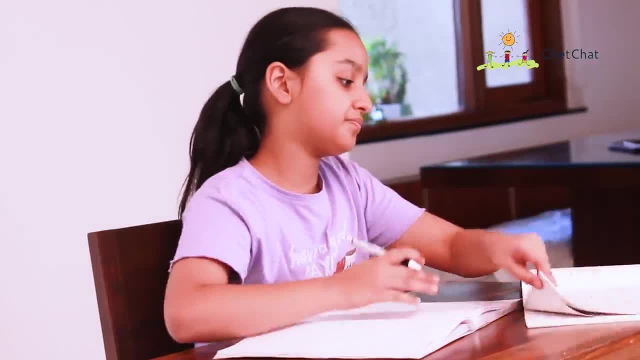 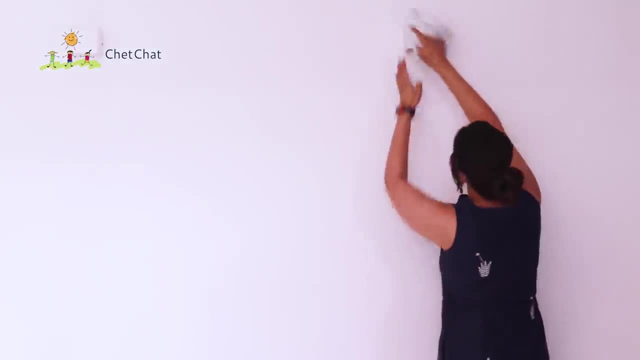 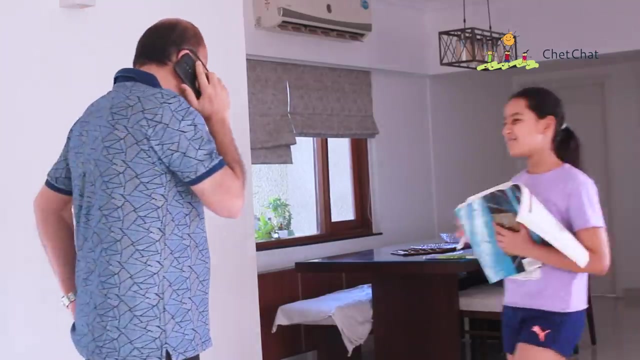 with the entire class. Now she stuck at home with her math book and confused with all kinds of questions. So Lavanya asked her parents to help her in math, But both of them were very busy with their office calls and household chores. Looking for a personal tutor at this stage was both 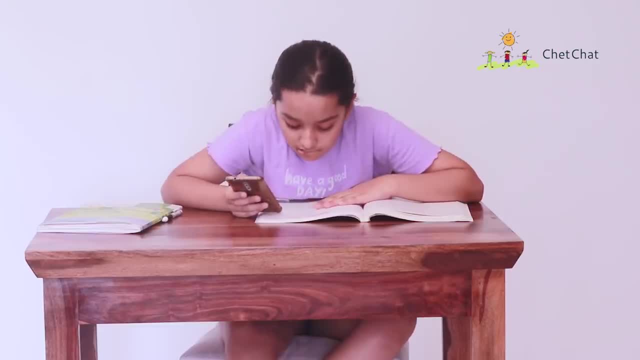 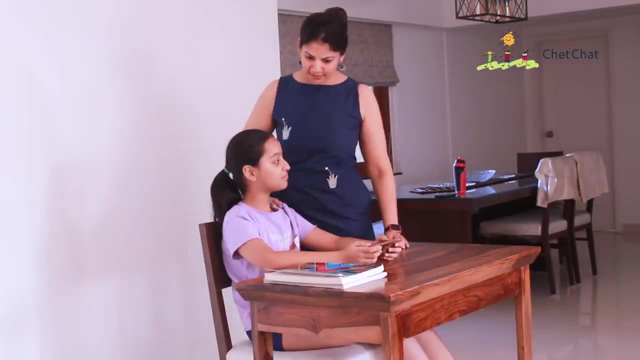 difficult and unaffordable, So she started surfing the internet for services. The teacher told her to look for solutions, But instead she kept getting distracted with games and comedy videos. Her mother bought her a membership to an online math course. Lavanya didn't find it helpful either. 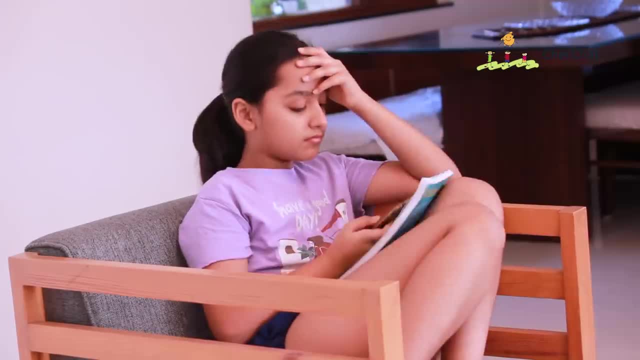 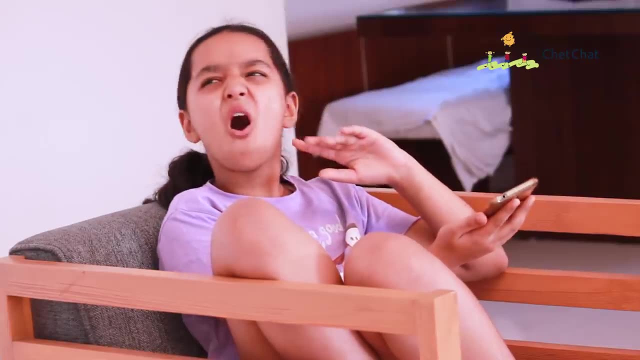 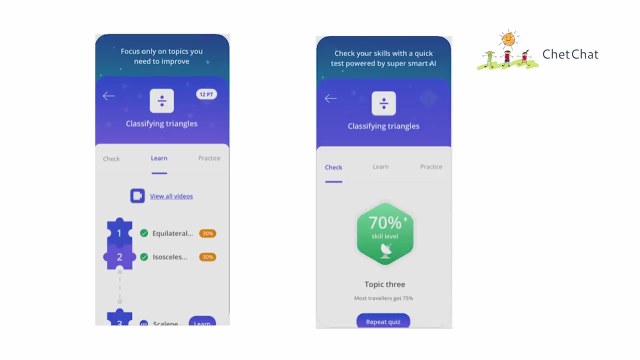 since it followed a pre-specified structure and syllabus for every user, It was not smart enough to understand her specific pain areas and it just didn't feel like a personal tutor. One day, her friend who was the topper of their class told her about the 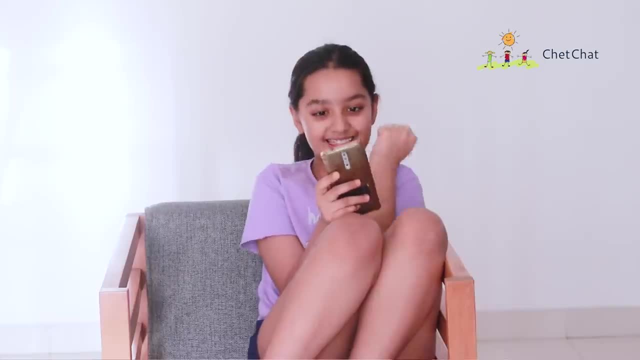 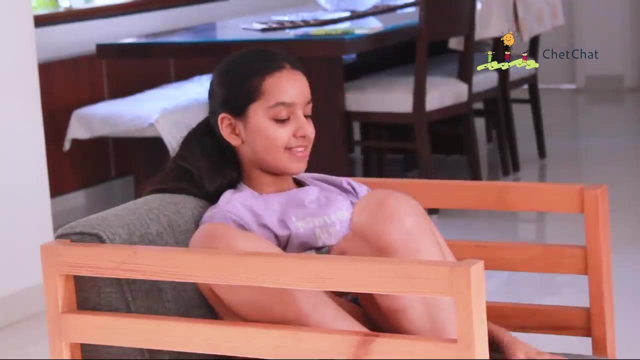 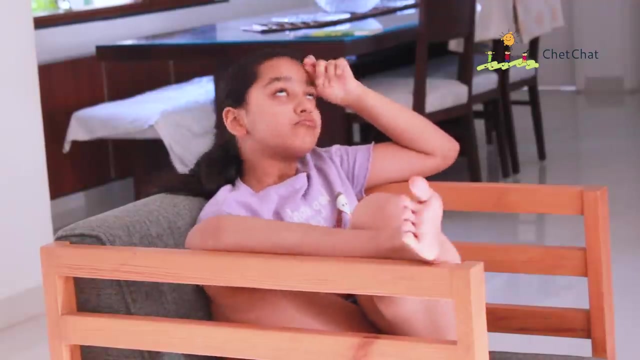 app Quickick by Pearson For Lavanya. it was love at first sight, since the app was very easy to use. It had tiny videos of less than two minute duration for every concept, And every time she answered a question wrong, somehow the app would find out what her real difficulty was And they would show. 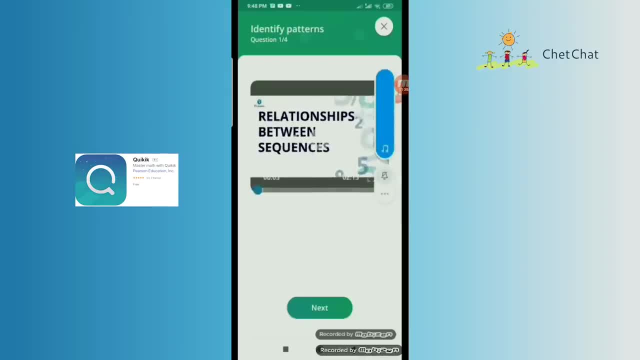 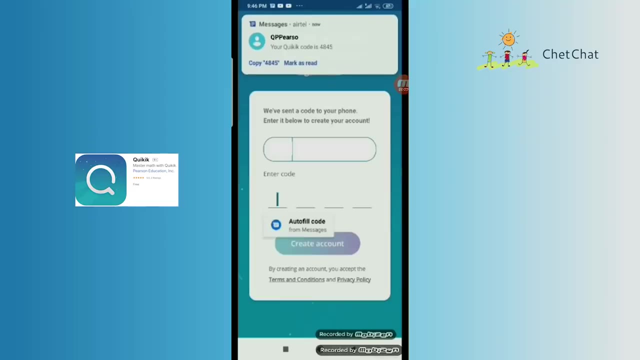 her short, bite-sized videos to help her solve her exact problem. It was like having a personal tutor who knew exactly what to tell you in two minutes without giving you a long lecture. She couldn't believe that this artificial intelligence embedded application was freely available. It takes just a few seconds to register and they don't even ask you for.